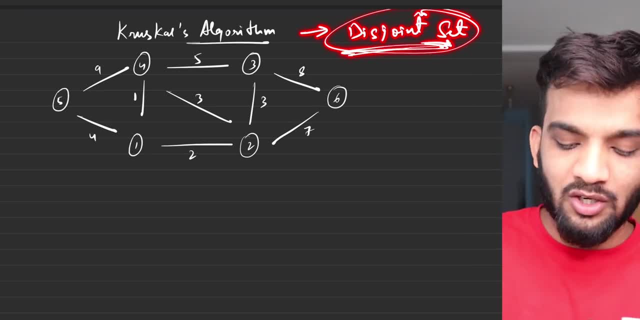 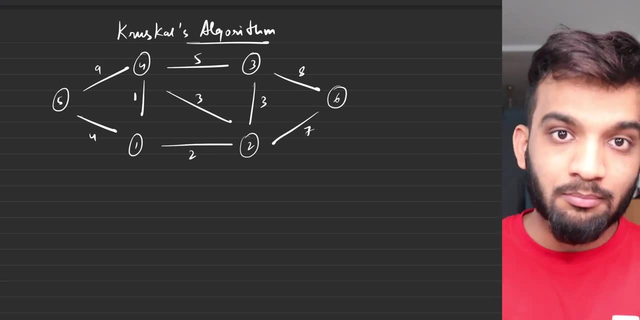 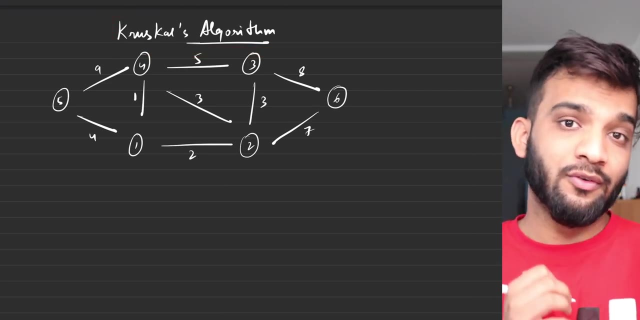 of clarity about the concept that will be used in order to solve the Kruskal's algorithm. If you do not know disjoint set, you will not understand anything. I'm assuming you have seen my disjoint sets video and then I'll be teaching you Kruskal's algorithm Right before this video. whichever you, 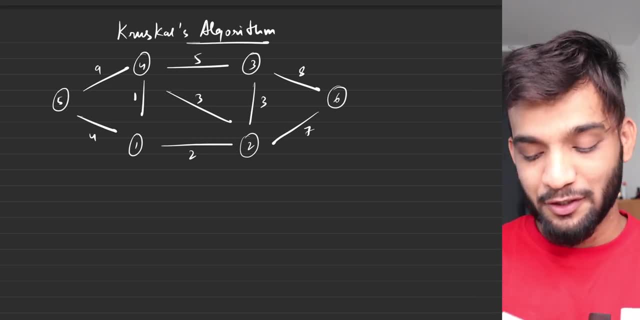 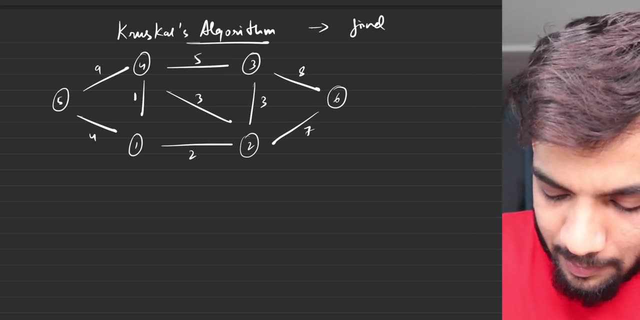 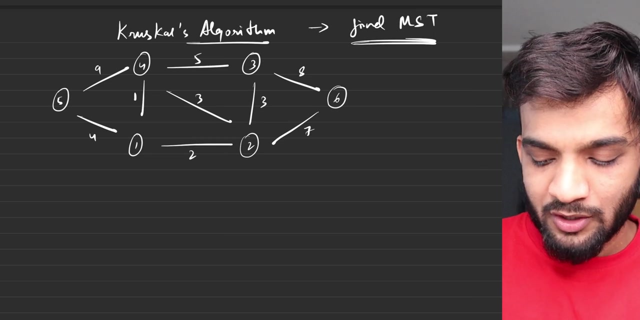 will find in the graph series is the Kruskal's, is the disjoint sets video. So what does Kruskal's algorithm help us to find? It helps us to find the minimum spanning tree. Now, what is a spanning tree? All of us know it. We have already discussed it in our previous lectures, right? So 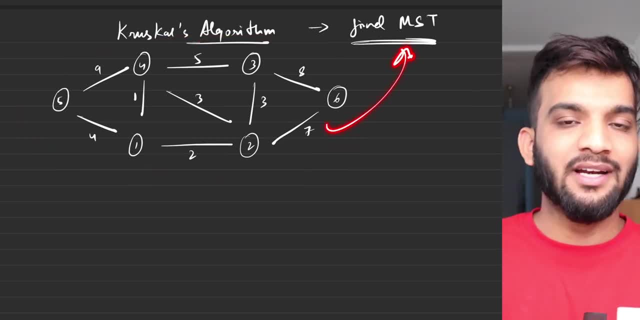 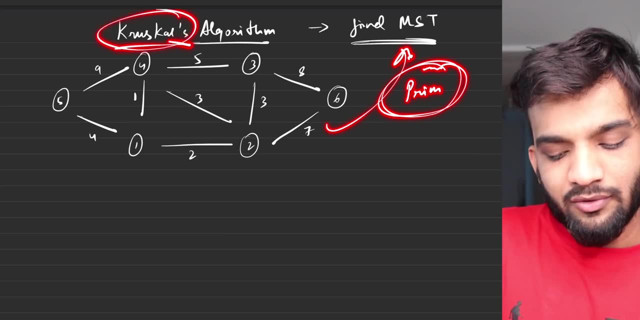 this is the given graph and you have to find the minimum spanning tree. We know we can implement Prim's algorithm to find it and we have done it in the previous videos, But in this video we will be applying the Kruskal's algorithm in order to find the minimum spanning tree of this particular. 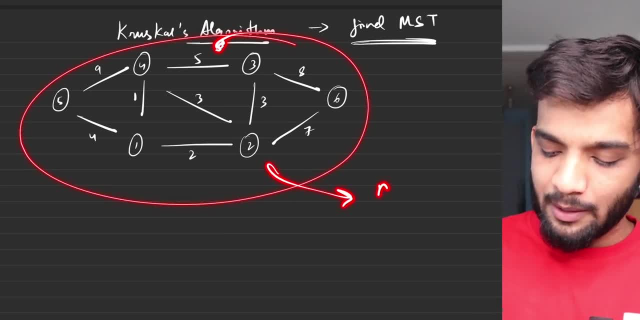 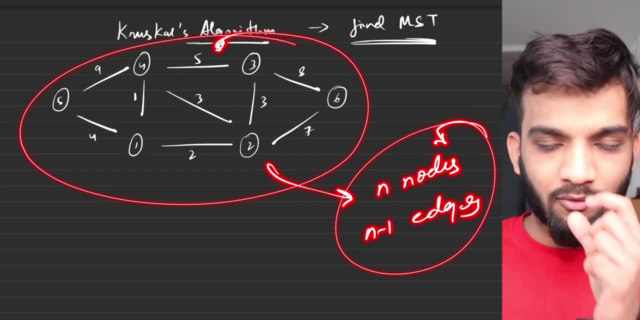 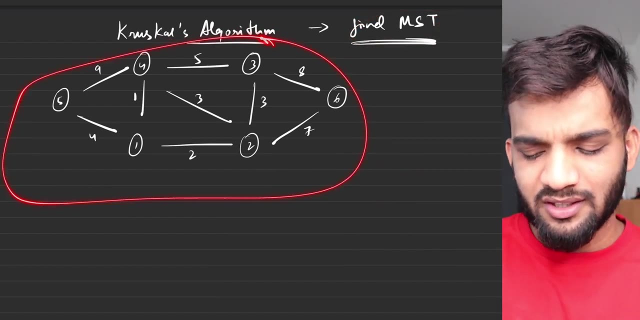 graph. What is the minimum spanning tree? If this graph can be represented in n nodes and n minus one edges, such that you can reach from one node to every other node, that is what you call as the minimum spanning tree. So you will be given a graph like this. You might be given the adjacency. 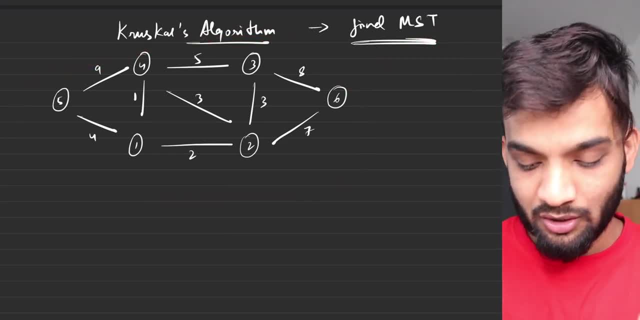 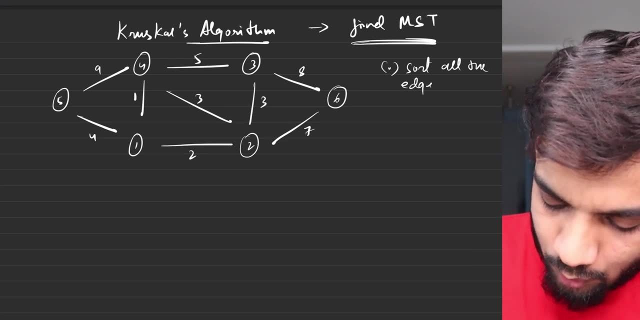 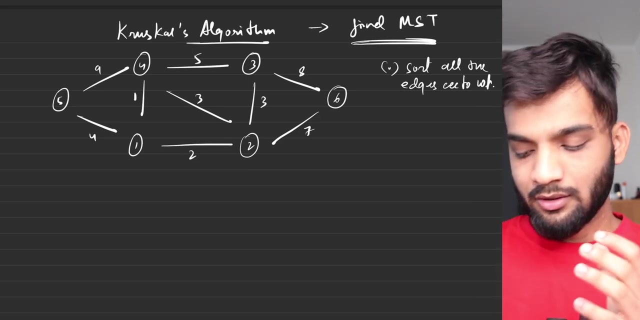 list. You might be given edges. You can be given anything. The first task that you need to do is sort all the edges. Remember this: Sort all the edges according to weight, Very, very important. According to weight. you have to sort all the edges. So let's quickly write down all the edges and 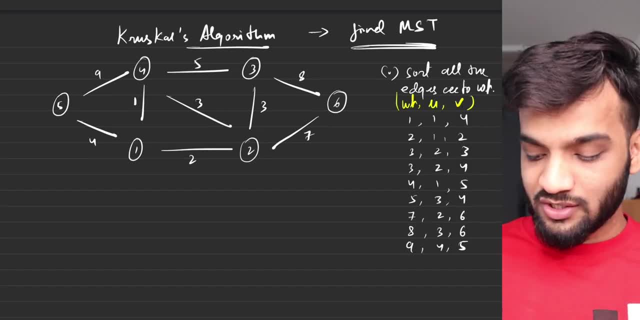 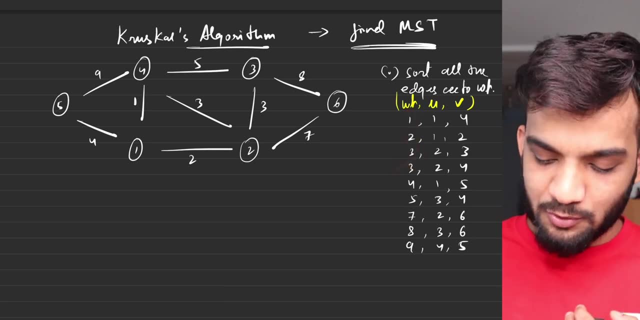 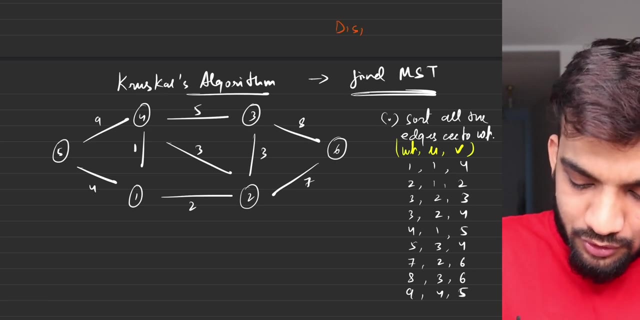 sort them according to weight. So, once you have sorted all the edges, you'll find all the edges like this And you see the minimum weight at the front and then the it keeps on increasing. Okay, so you know the data structure- disjoint set- that we are going to use. What does disjoint set provide? 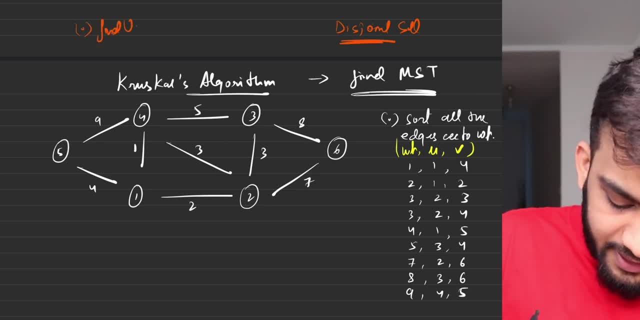 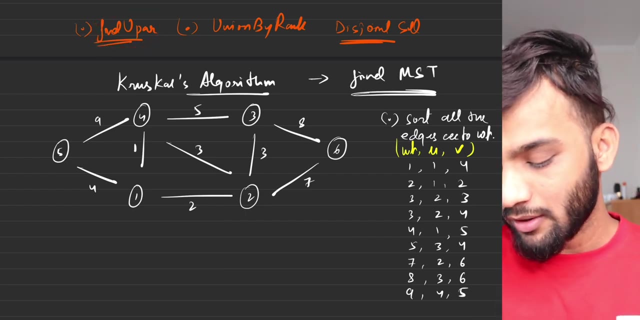 us with. It provides us with two things: Find ultimate parent. and it also provides us with union by rank And we know if two guys belong to the same component, they will always have the same ultimate parent of the boss, right? So remember initially when you declare the disjoint. 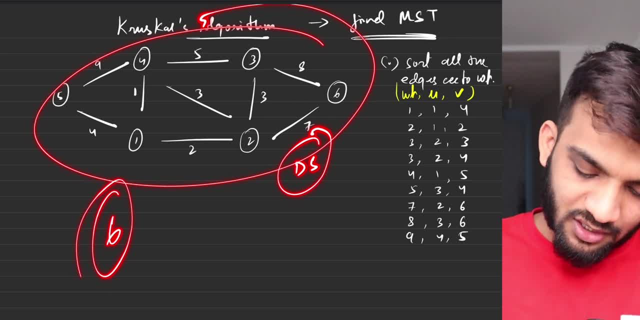 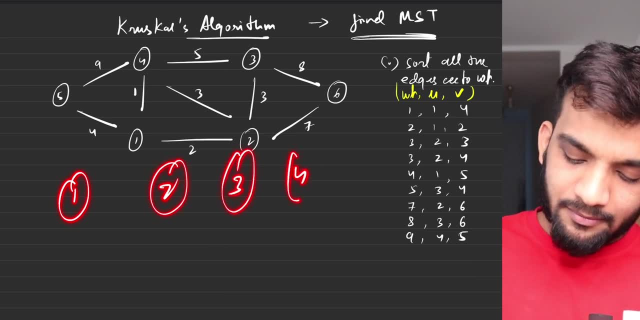 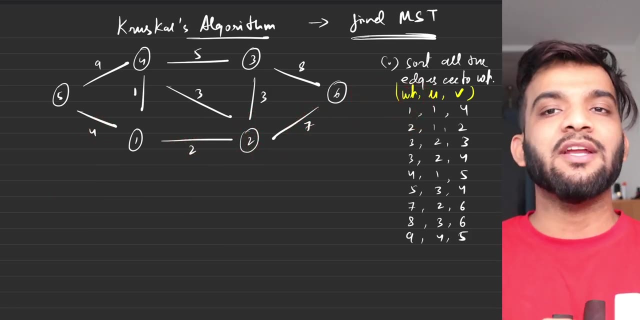 set with all these nodes. So over here we have six nodes. if you carefully observe, If you define a disjoint set with six nodes, everyone will be a single guy. Everyone will be a single guy with the parent pointing to themselves. So everyone is single with the parent pointing to themselves. So 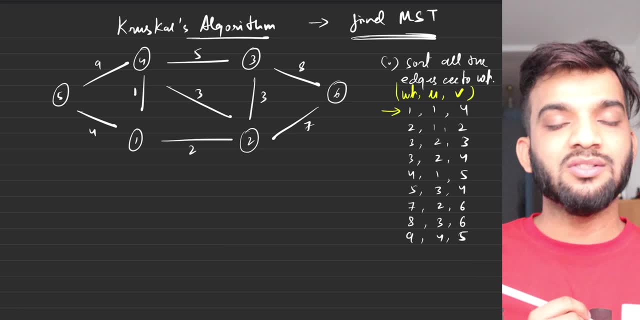 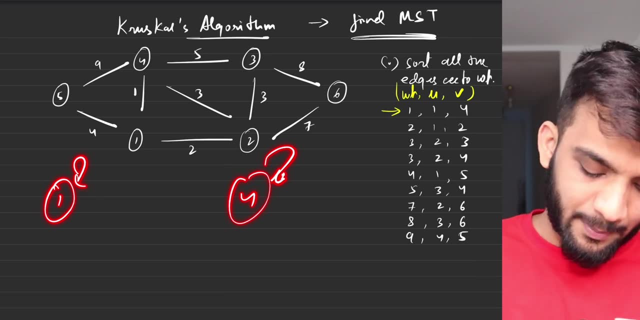 the first node is what you take. So let's quickly take the first node, which is saying 1 comma 4. so you say: okay, 1, 4, 4 is your ultimate parent. 1 says 1, 4 says 4, so do they? 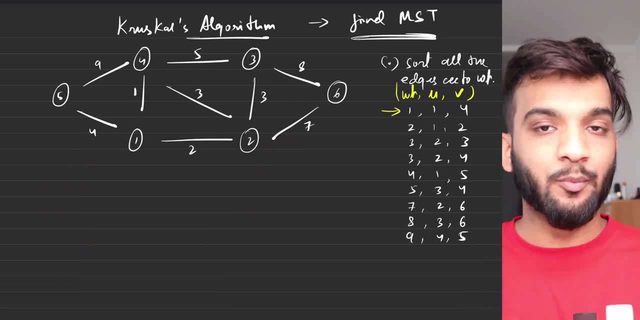 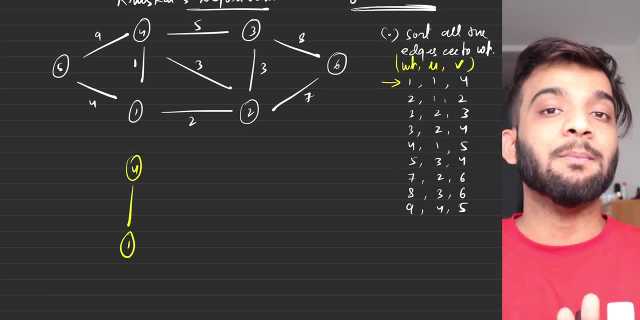 belong to the same component. no, they do not belong to the same component. so what you will do is you will go ahead and say, okay, since they do not belong to the same component, i can take it, and this will be part of my mst, because this is the most minimal edge in the graph, so let's take it. 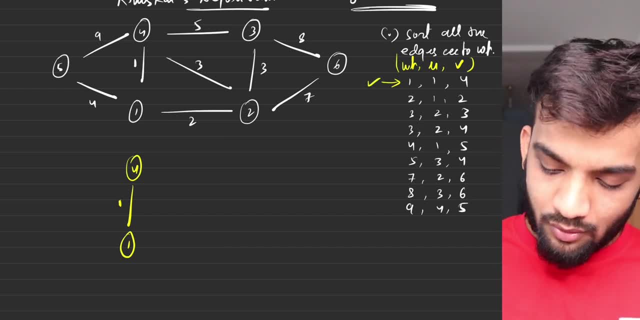 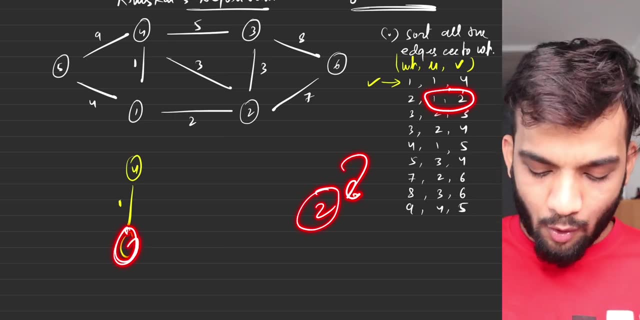 right, so i've taken it perfect. next is 1 comma 2. so you have a 1 and you have a 2, so 2's parent is himself and 1 is this component. do they belong to the same component? again, this joint set will: 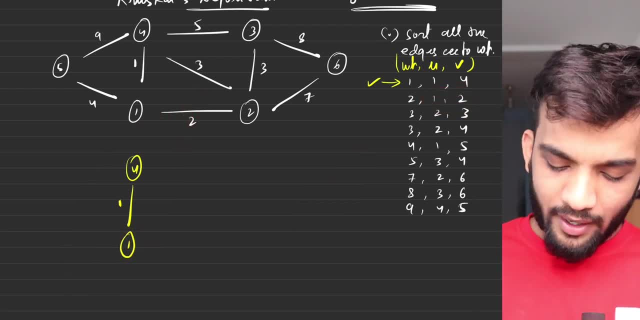 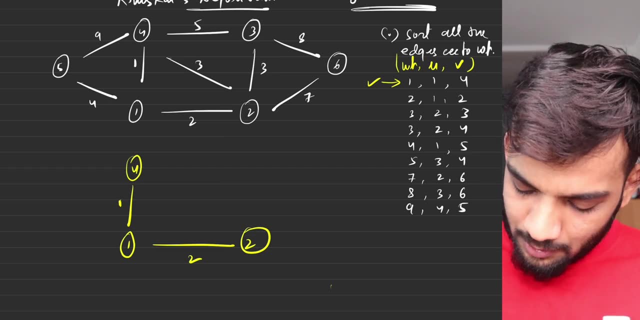 say you know they do not belong to the same component. so you will go ahead and update 1 comma 2 with the edge. so this will also be a part of your mst and you can also keep on counting the weight. the weight will be 1 plus 2 because there are two edges which have been 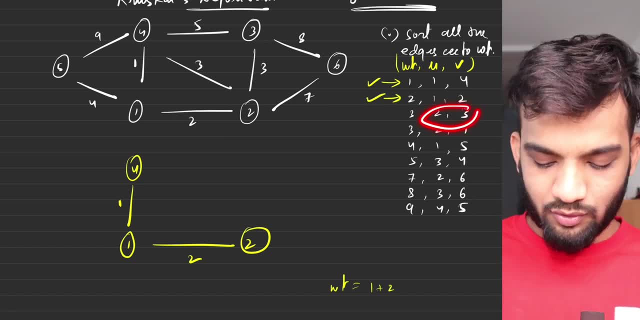 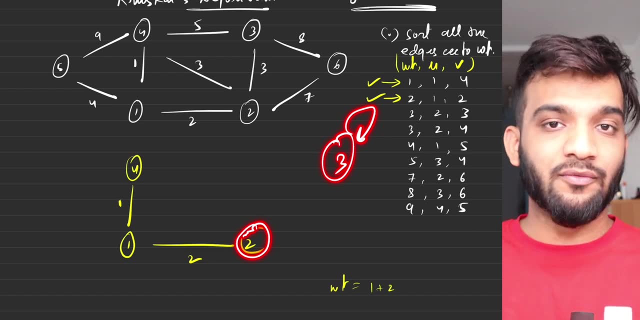 added. so this is done. next is 2 comma 3. this time there is 2, who will have an ultimate parent, and there is 3, who will have an ultimate parent as 3 itself. 3 has the ultimate parent as itself and 2 is here in this component. they definitely do not belong to the same component, so you can. 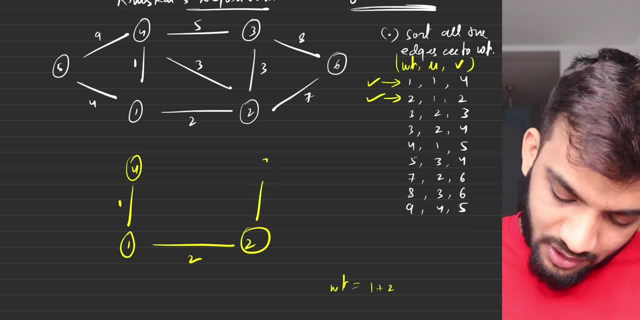 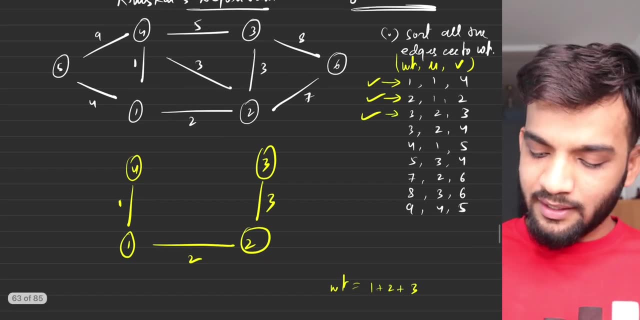 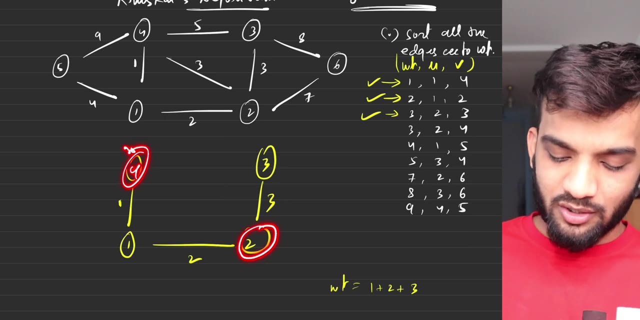 go ahead and add 3. yes, you can go ahead and add 3 into your mst as well, and that will be the edge weight. perfect, this is also done, which is the next one. the next one is 2 comma 4. now, this time, when you try to find the ultimate parent of 2 and 4, they will come out to be the same, because they belong to a same component, so you'll be like: i will not take this into my mst because they are already connected. this will not make sense because you can all already reach everyone, like every node can be reachable to every other node. so what's the point of making a cycle and introducing an extra? 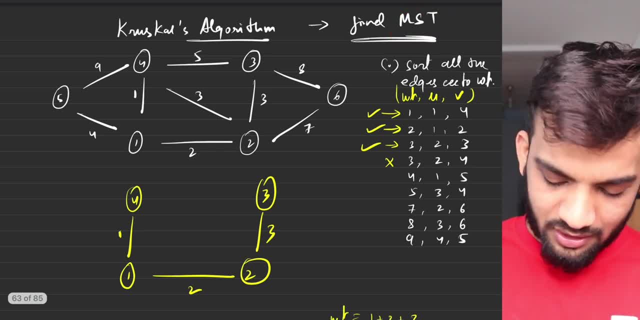 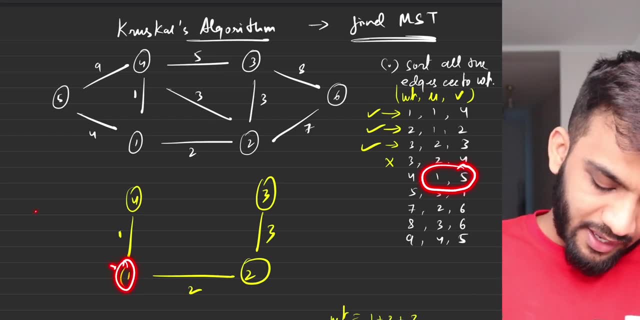 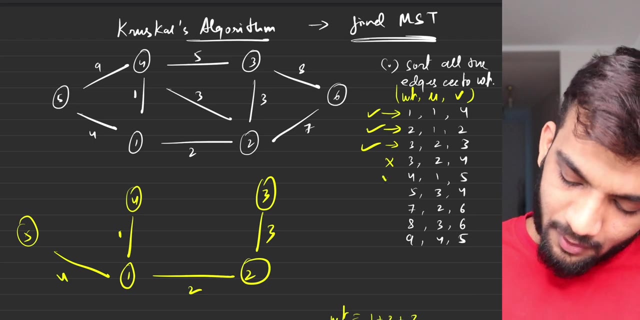 edge because our goal is to find minimum, so including an extra edge will not help us right. so we have 2 comma 5. so 1 is here and 5 is a single guy. again, they do not belong to the same component. this joint set will help you to find this, so go ahead and add this. perfect, what's the? 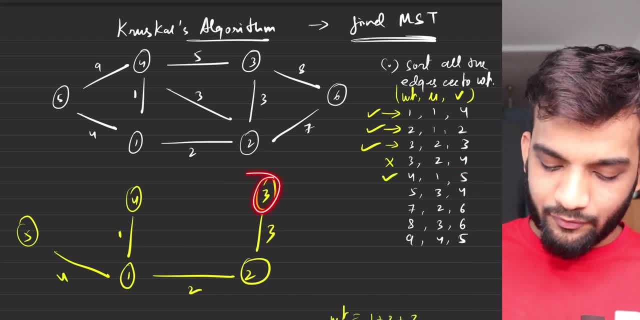 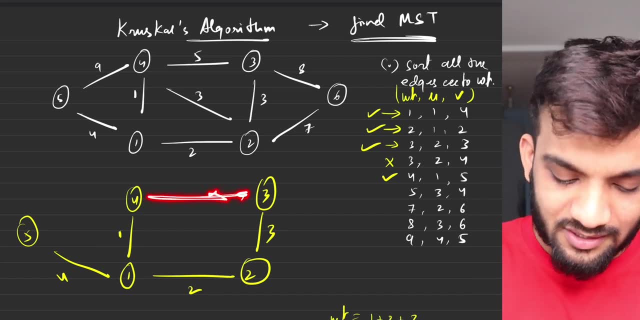 next thing? the next thing is 3 comma 4, so we have a 3, we have a 4 and they definitely belong to the same component. this joint set will again help you to find this. so you'll not add this, because there's no point in adding this. we'll go ahead and discard it. next you have 2 comma 6, so you have a 2 over. 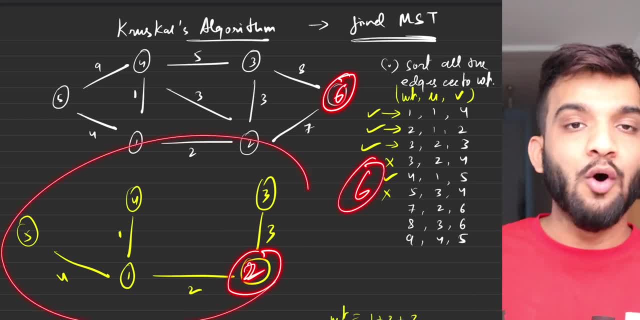 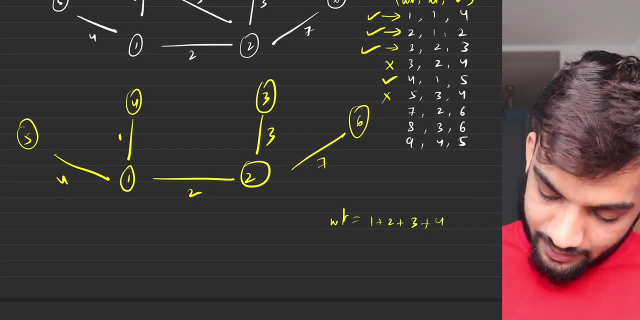 here and you have a 6 over here alone, and 2 is a part of this component, so you can go ahead and say, okay, i'll take up 6 and that will be 7.. so, by the way, i forgot to write 4 and now 7. yeah, so this will be a part of it. what's the next? 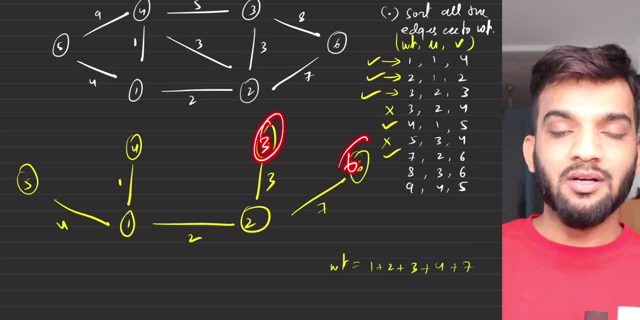 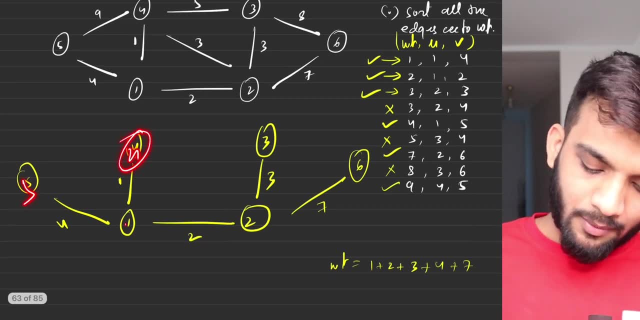 it's 3 comma 6 whereas 3 whereas 6. they belong to the same component, so not to be taken. what's the next? 4 comma 5? so the 4 and 5 belong to the same component, so again i will end up not taking it. 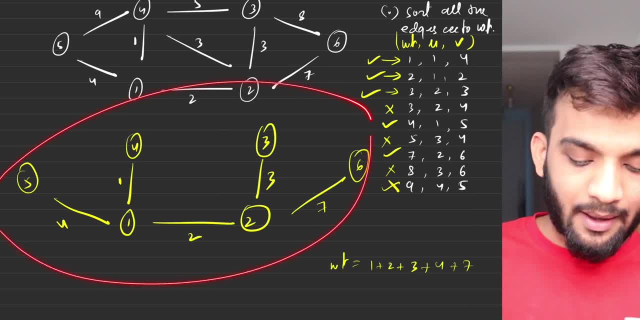 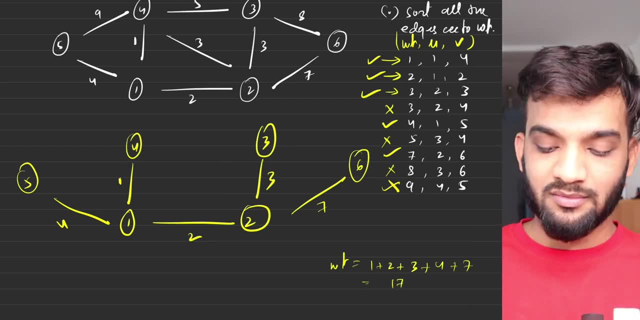 so apparently i can say: this is, this is my mst, and the summation of weights will be 1 plus 2, 3 plus 3, 6, 10, 17 is the summation of weights? very simple, isn't it? you just need to know this joint set. 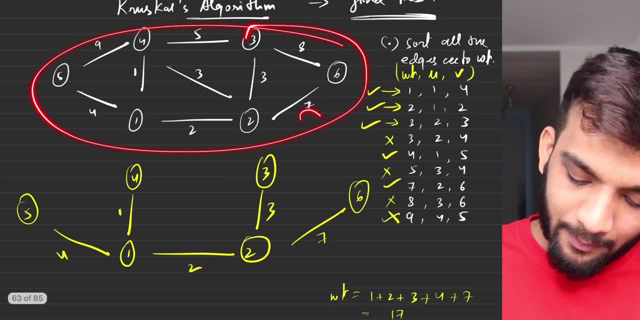 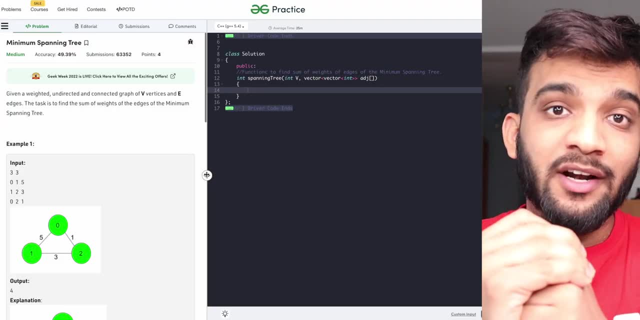 data structure, and you can easily find mst from any given graph. the weight as well, as well as the mst got it. so, guys, i hope you have understood the entire explanation of triskel's algorithm. now it's time to code it up. so, as usual, the c plus plus solution is on the right and the 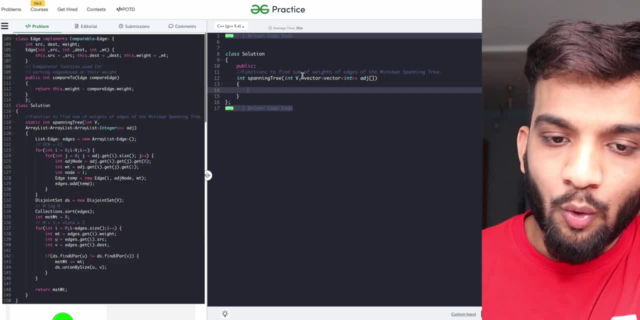 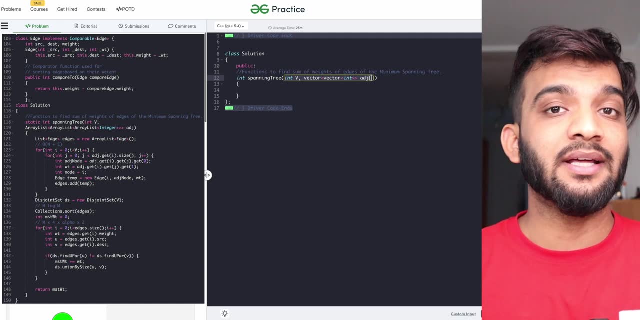 exact, similar java code will be on the left of the java people. so what are we given? we're not given the edges. we are rather given an adjacency list. and remember, it's an adjacency list, so it will be containing the graphs in bi-directional edges, like if you look at the driver code as well. 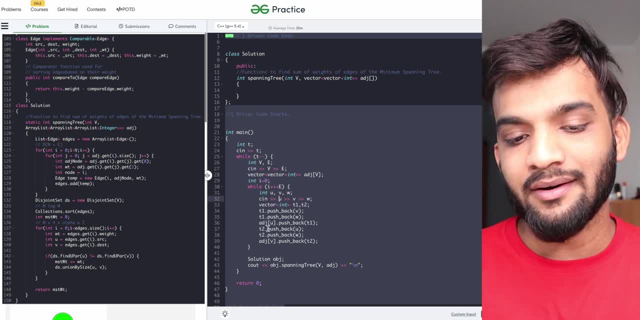 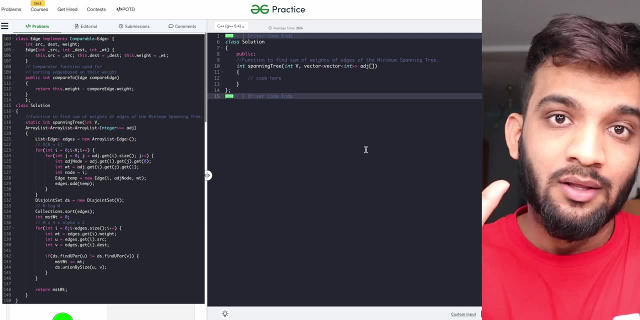 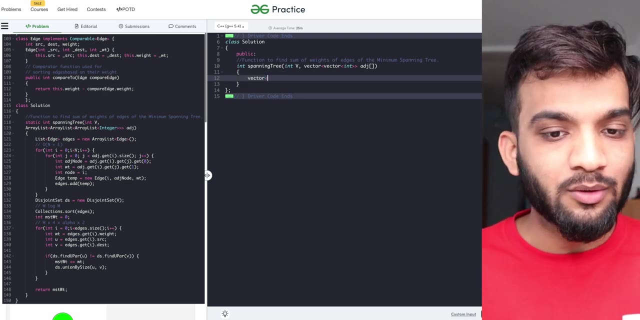 they're basically taking the edge with uvw and they're basically storing it in two versions, carefully see. so since it is a bi-directional edge, it will be stored in two ways. so it's, it's pretty simple. uh, no need to panic. so, since we are storing a tuple, what you can do is you can say: 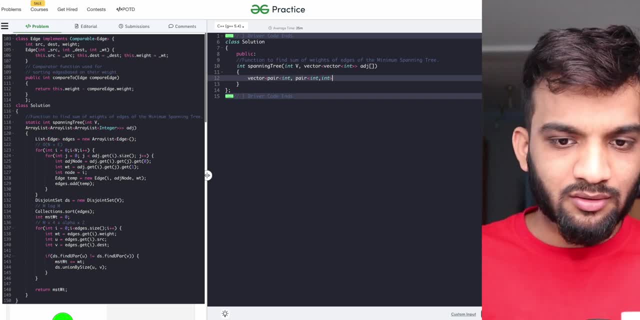 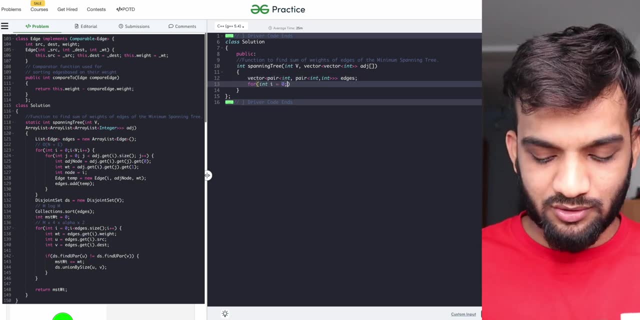 okay, vector of pair. this will be the weight, and then i'll go ahead and store the two other nodes. so this will be my edges where i'll be storing. now i will be going across all the nodes. yes, i'll be going across all the nodes. so let's, it's a zero based indexing and it's absolutely no problem. 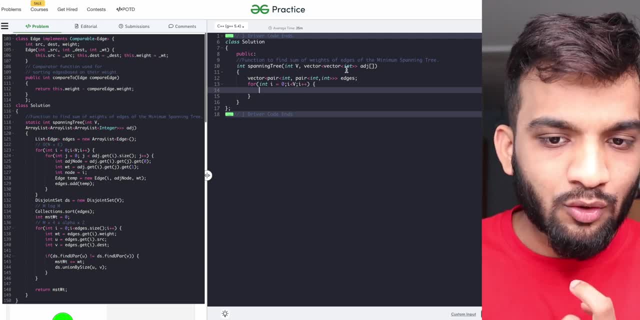 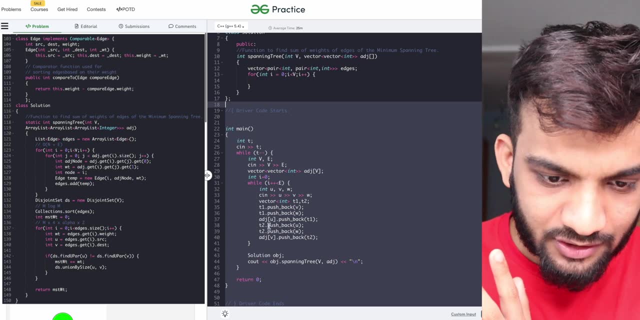 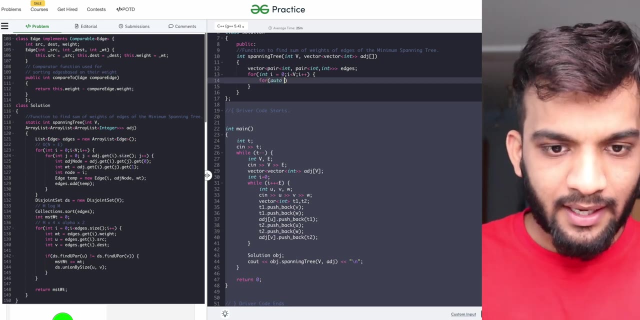 so i'll be going across all the roots. right now, in every node they're storing a vector which is basically storing the- if you look at the driver's code again, basically storing u and w, basically the adjacent node and the weight. so i can go ahead and say okay. 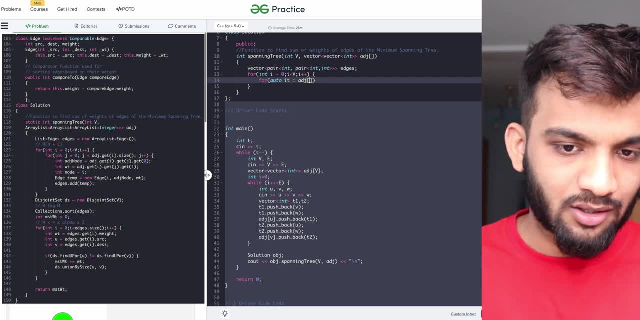 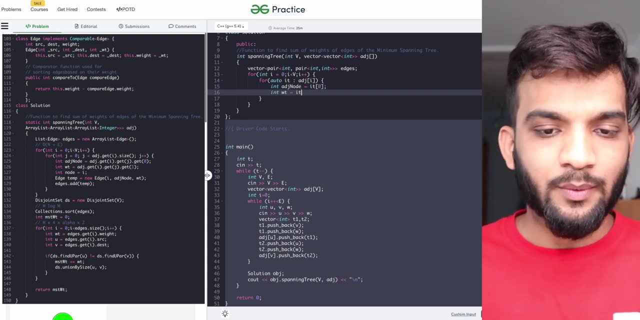 i'll go ahead with this. adjacents of i and i can get the adjacent node which will be at the id of 0. i'll get the weight which will be at id of 1, right, and i know the node is nothing but the i. 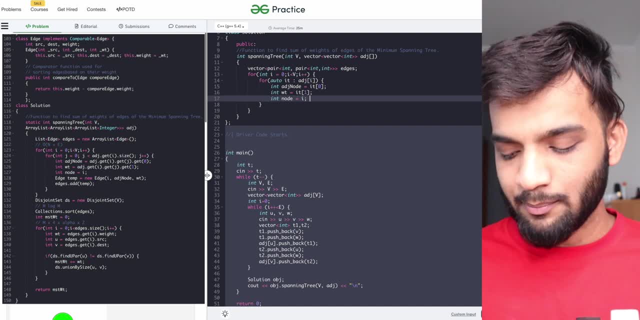 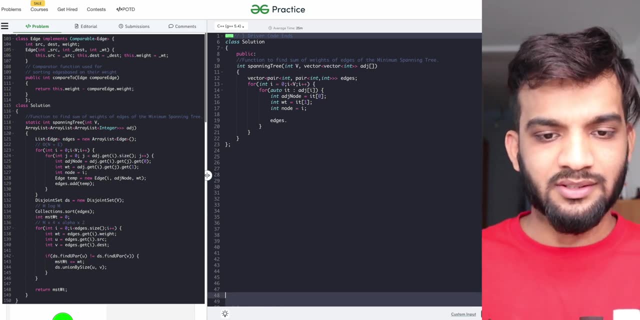 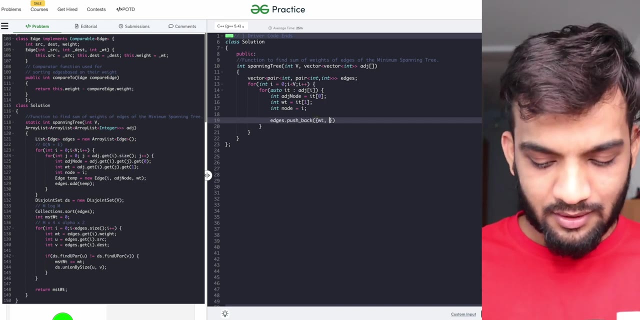 correct. i know the node is nothing but the i just, in order to improve understanding, i've written it. so can i say edges? can i say edges is maybe i'll just remove this clearing, okay? maybe i can say: edges, dot, push back. what should i say? i say: wait, i know it's from node to adjacent node. perfect, now you might see, but striver, since it's a. 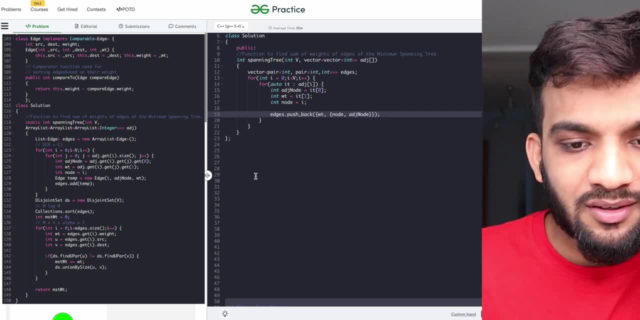 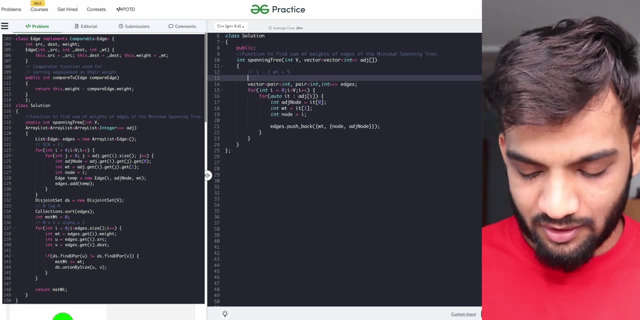 if there is an edge between 1 to 2 with a weight of 5, then one at one, there will be two comma five. one at one, there will be two comma five. one at one, there will be two comma five, like on the adjacency list. on one, you will have two. 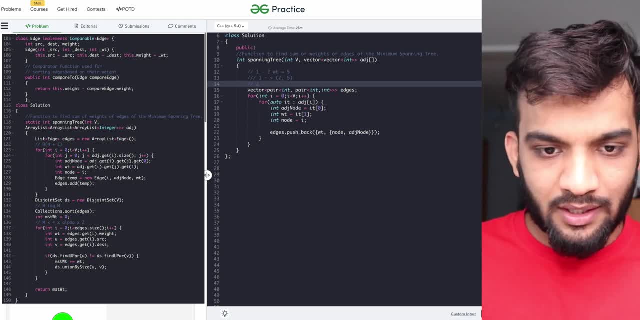 like on the adjacency list, on one, you will have two. like on the adjacency list, on one, you will have two comma five. and even at the place of two, you comma five. and even at the place of two, you comma five. and even at the place of two, you will have, if you remember, the artist. 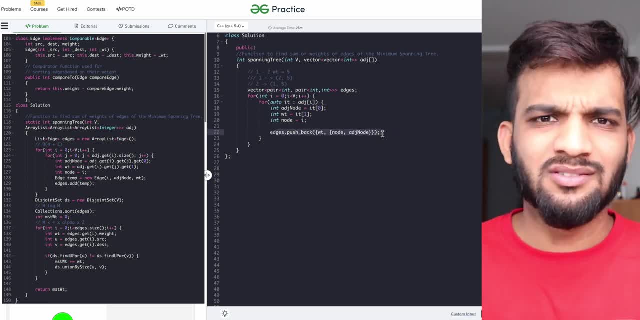 will have. if you remember the artist will have, if you remember the artist, one comma five. so you'll apparently insert one comma five. so you'll apparently insert one comma five. so you'll apparently insert two edges. it is okay, we're using disjoint two edges. it is okay, we're using disjoint. 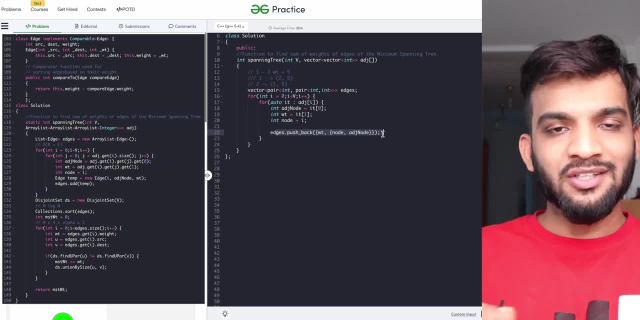 two edges. it is okay. we're using disjoint set, it will automatically discard it. if set, it will automatically discard it. if set, it will automatically discard it. if you've taken one edge, it will automatically. you've taken one edge, it will automatically. you've taken one edge, it will automatically discard the next stage, right so? 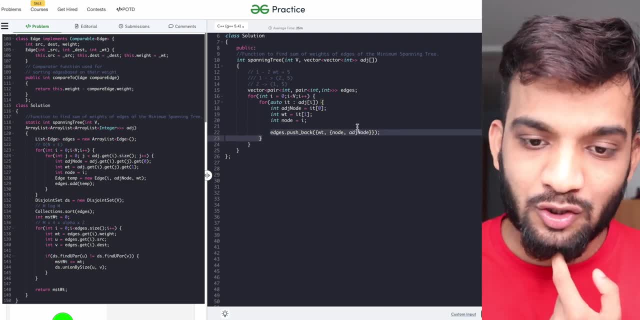 discard the next stage right. so discard the next stage right. so it definitely goes ahead and adds: it definitely goes ahead and adds. it definitely goes ahead and adds twice this edge like one. it will add twice this edge. like one, it will add twice this edge. like one. it will add is: 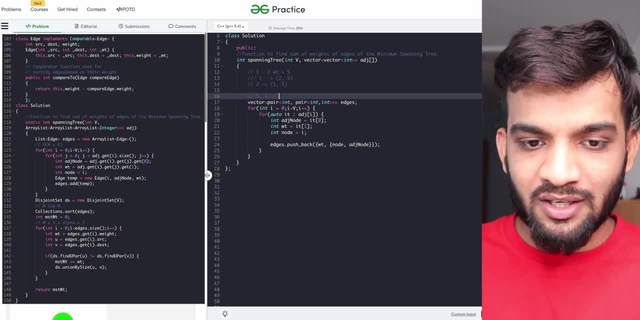 is is first time it will add is five comma one. first time it will add is five comma one. first time it will add is five comma one to two edge, and then the second time it to two edge, and then the second time it to two edge, and then the second time it will add as five comma two comma one. so 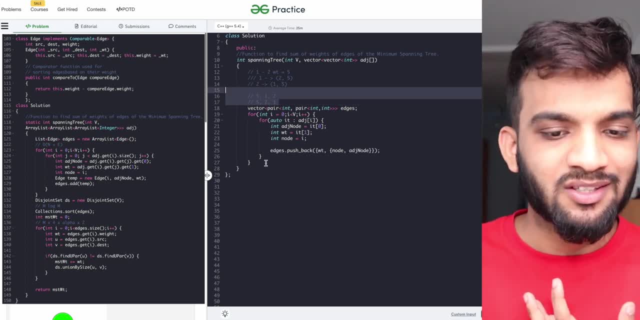 will add as five comma two comma one. so will add as five comma two comma one. so it'll definitely add twice. but that is, it'll definitely add twice, but that is, it'll definitely add twice. but that is none of my concern because we are using. none of my concern because we are using. 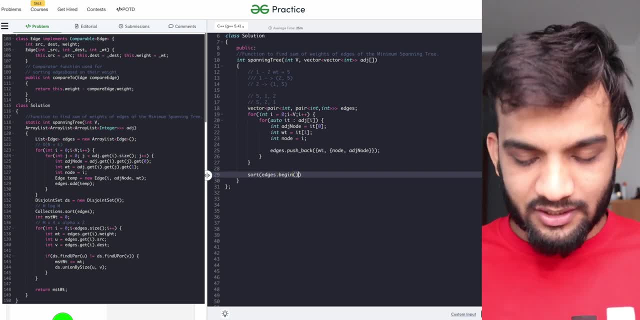 none of my concern, because we are using a data structure which is going to a data structure which is going to a data structure which is going to ignore it. so edges dot begin. ignore it. so edges dot begin. ignore it. so edges dot begin. edges dot end. edges dot end. 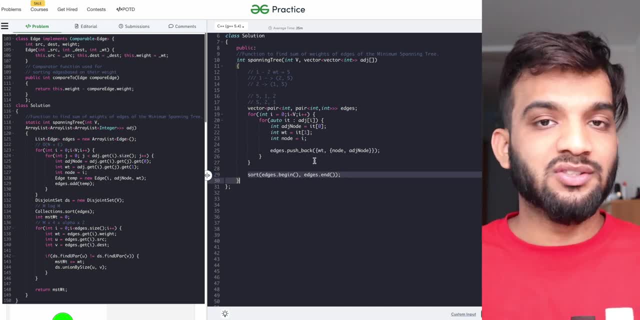 edges dot end: right, right, right, perfect. we have sorted the edges. now we perfect, we have sorted the edges. now we perfect, we have sorted the edges. now we need a data structure, for sure, but before need a data structure, for sure, but before need a data structure, for sure, but before that, let's see what else we need. we need: 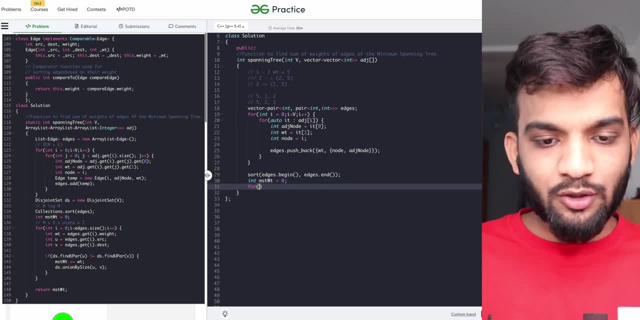 that. let's see what else we need. we need that. let's see what else we need. we need to find the mst weight. so maybe mst to find the mst weight. so maybe mst to find the mst weight. so maybe mst weight will be zero and we need to go. 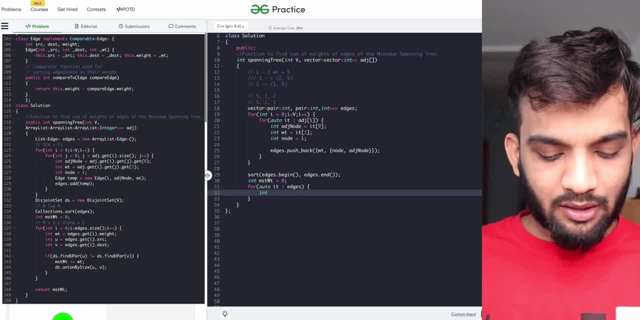 weight will be zero and we need to go. weight will be zero and we need to go across all the edges. so let's quickly across all the edges. so let's quickly across all the edges. so let's quickly uh find the weight. weight will be at. uh, find the weight, weight will be at. 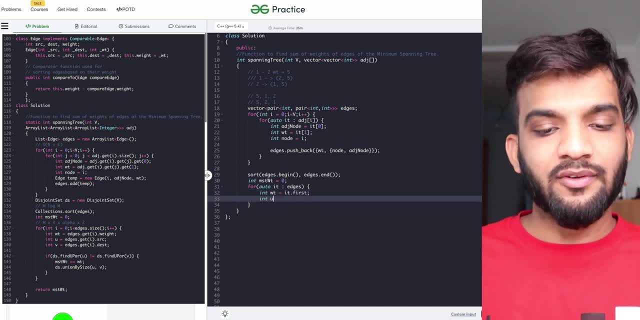 uh, find the weight. weight will be at id, dot, id, dot, id, dot, first, first, first, and then we will have a u, which will be, and then we will have a u, which will be, and then we will have a u, which will be id, dot, second, dot. first we will be having 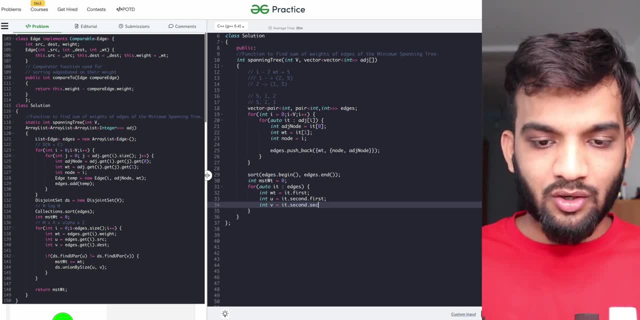 id dot, second, dot first. we will be having id dot, second, dot first. we will be having a view which will be uh v, rather a view which will be uh v, rather a view which will be uh v, rather, it dot, second, dot, second and then going. it dot, second, dot, second and then going. 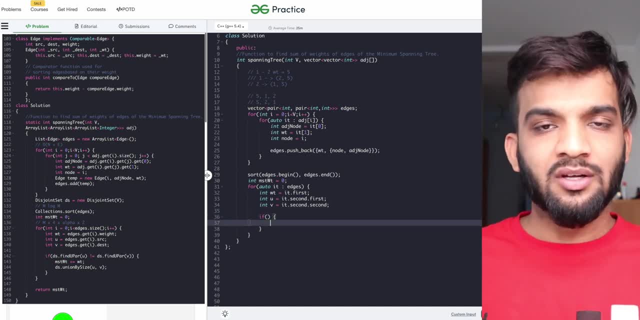 it: dot, second, dot, second and then going ahead. we need to figure out if they ahead. we need to figure out if they ahead. we need to figure out if they belong to the same component or not. belong to the same component, or not belong to the same component or not. this we will implement the data. 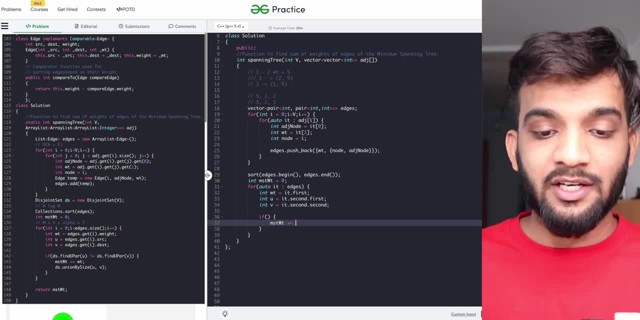 this we will implement the data. this we will implement the data structure. and if they belong to the like structure. and if they belong to the like structure, and if they belong to the like, if they do not belong to the same data, if they do not belong to the same data. 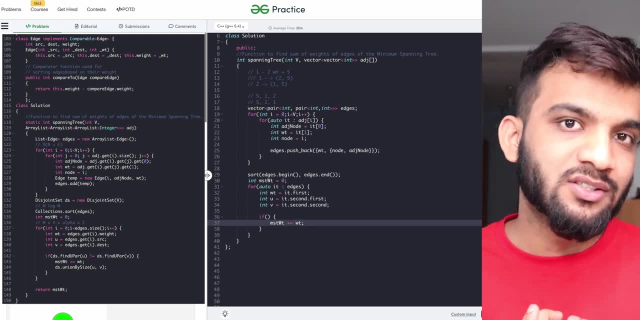 if they do not belong to the same data structure, we will take the weight and structure. we will take the weight and structure. we will take the weight and add it. if they would have asked us to add it, if they would have asked us to add it, if they would have asked us to store mst, we can. 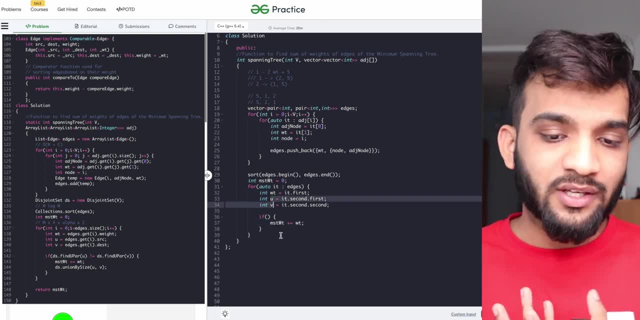 store mst. we can store mst, we can. we know the edges between u and v. you, we know the edges between u and v. you, we know the edges between u and v. you can also store the mst, but over here. can also store the mst, but over here. 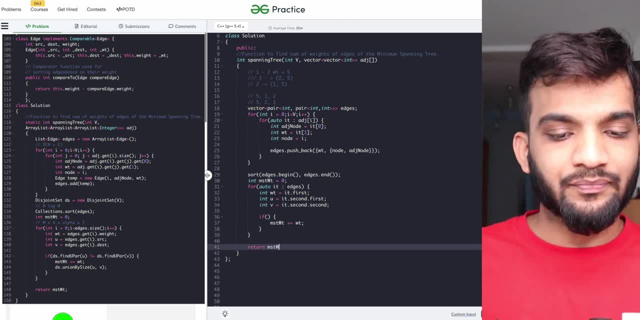 can also store the mst, but over here they just need the mst weight, so i'll go. they just need the mst weight, so i'll go. they just need the mst weight, so i'll go ahead and return the mst. ahead and return the mst. 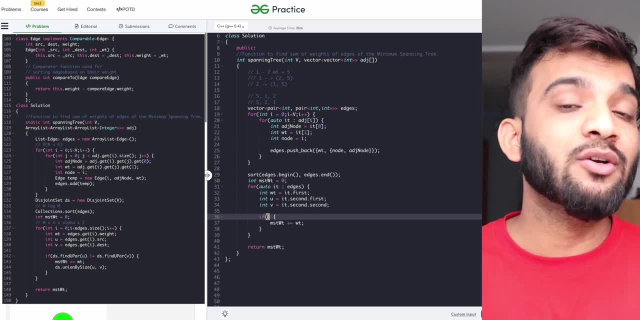 ahead and return the mst wait. but now, how do you figure out if wait? but now, how do you figure out if wait? but now, how do you figure out if they're belonging to the same component? they're belonging to the same component. they're belonging to the same component, it or not. if you remember, we have 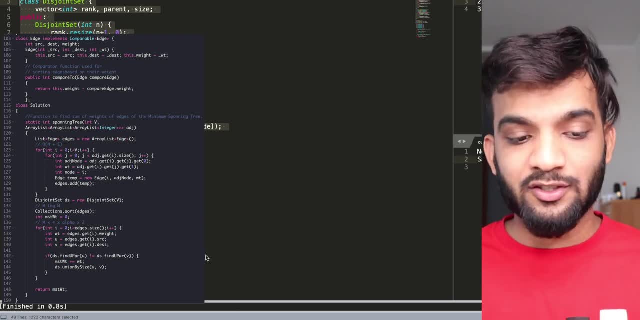 it or not. if you remember, we have it or not. if you remember, we have already discussed something uh like. already discussed something uh like. already discussed something uh like disjoint set data structure and this disjoint set data structure and this disjoint set data structure. and this was the snippet of code, so just copy. 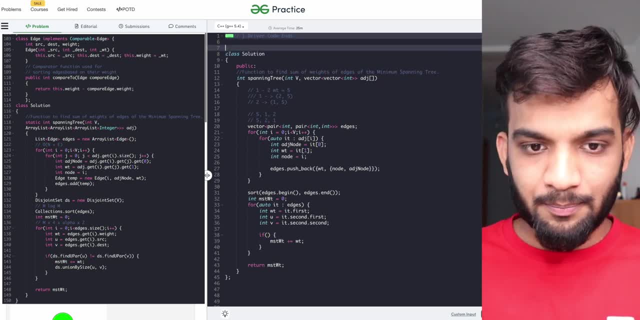 was the snippet of code, so just copy was the snippet of code, so just copy. paste and i'll go to the solution. yes, paste and i'll go to the solution. yes, paste and i'll go to the solution. yes, and i'll paste this class. so i have this. 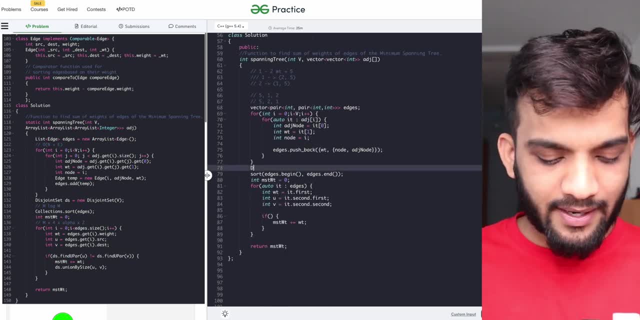 and i'll paste this class. so i have this and i'll paste this class. so i have this. disjoint set data structure already ready. disjoint set data structure already ready. disjoint set data structure: already ready with us. so i'll go ahead and declare with us. so i'll go ahead and declare. 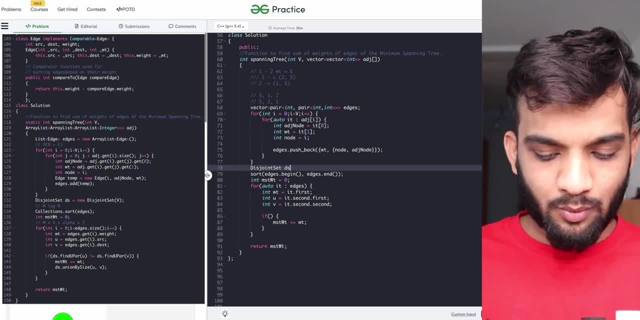 with us. so i'll go ahead and declare disjoint, disjoint, disjoint. set ds with v vertices done, i'll say ds. set ds with v vertices done, i'll say ds. set ds with v vertices done, i'll say ds. can you find the ultimate parent? because? can you find the ultimate parent? because 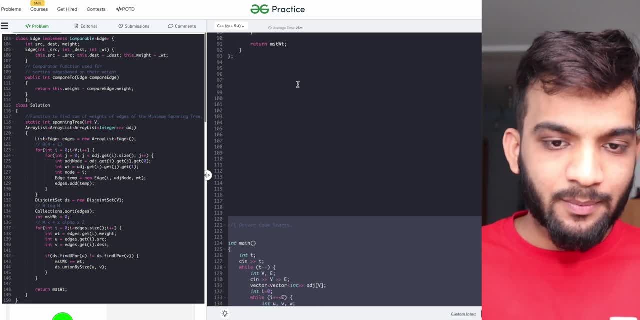 can you find the ultimate parent, because this is the function. if you see this is the function, if you see this is the function, if you see find ultimate parent, so i will be like find ultimate parent, so i will be like find ultimate parent. so i will be like, okay, cool, can you find me the ultimate? 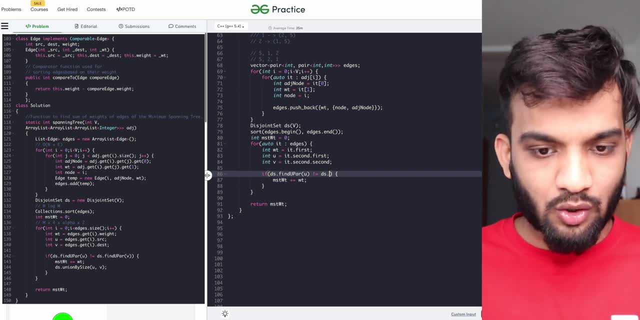 okay cool, can you find me the ultimate? okay cool, can you find me the ultimate parent of you? parent of you. parent of you. if that's not equal to ds dot find. if that's not equal to ds, dot find. if that's not equal to ds, dot find the ultimate parent of you. that means they: 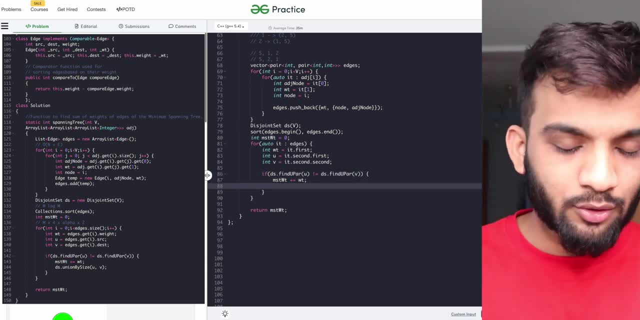 the ultimate parent of you. that means they the ultimate parent of you. that means they belong to the different component, belong to the different component, belong to the different component. so i'll go ahead and take it to the mst. so i'll go ahead and take it to the mst. 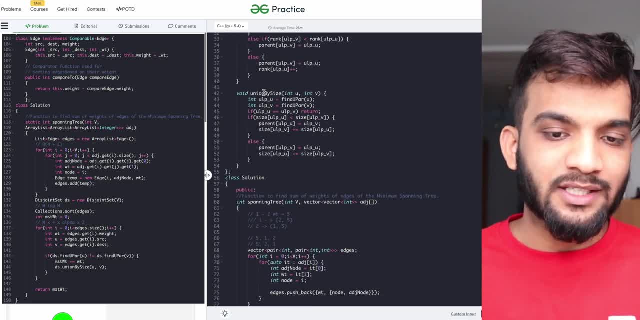 so i'll go ahead and take it to the mst. at the same time i'll say you can use. at the same time i'll say you can use. at the same time, i'll say you can use union by rank or union by size, whichever- union by rank or union by size, whichever. 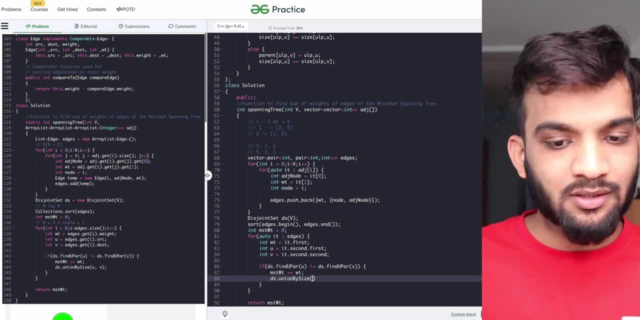 union by rank or union by size, whichever you, you you wish to, you can go ahead and say union by wish to. you can go ahead and say union by wish to. you can go ahead and say union by size, size, size, and you'll go u comma v. that's it, you. 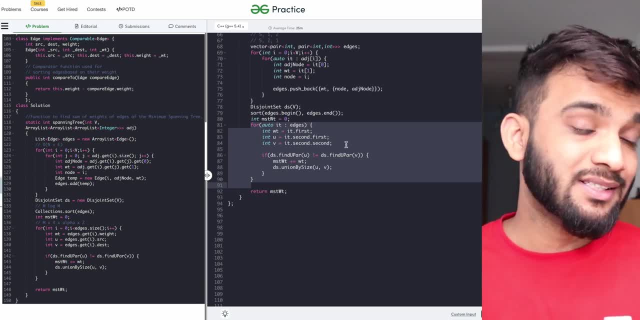 and you'll go u comma v, that's it. you and you'll go u comma v, that's it. you make it a union simple as that now. i'll make it a union simple as that now. i'll make it a union simple as that. now i'll go ahead and compile and see if it is. 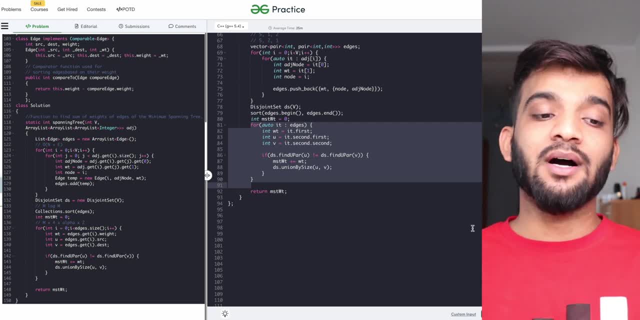 go ahead and compile and see if it is. go ahead and compile and see if it is running, running, running. fine, indeed, it is now. let's quickly, uh, fine, indeed, it is now, let's quickly, uh fine, indeed, it is now, let's quickly, uh, submit this and see if it is giving us. 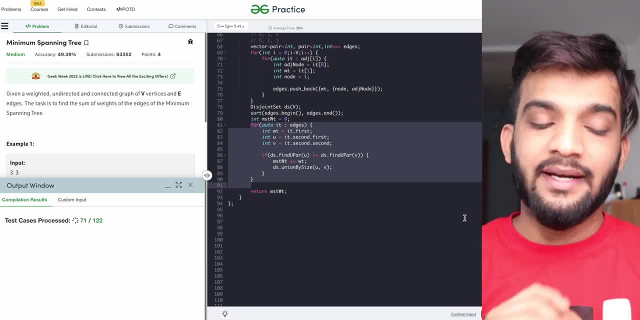 submit this and see if it is giving us submit this and see if it is giving us correct answers or not. it is indeed running for all the test. it is indeed running for all the test. it is indeed running for all the test: cases, cases, cases. yes, it is. so now we've understood most. 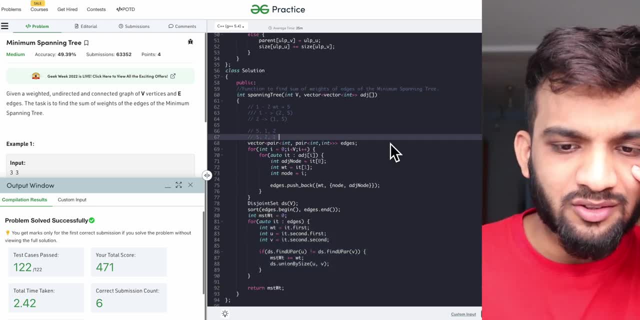 yes, it is so now we've understood most. yes, it is so now we've understood most of the algorithm. what about the time of the algorithm? what about the time of the algorithm? what about the time? complexity first? uh, you're figuring out. complexity first- uh, you're figuring out. 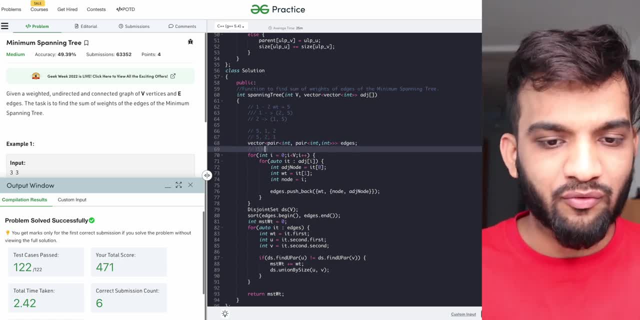 complexity first. uh, you're figuring out all the edges. so this is definitely all the edges. so this is definitely all the edges. so this is definitely going to take a bigo of n plus the going to take a bigo of n plus the going to take a bigo of n plus the number of edges, because you're going. 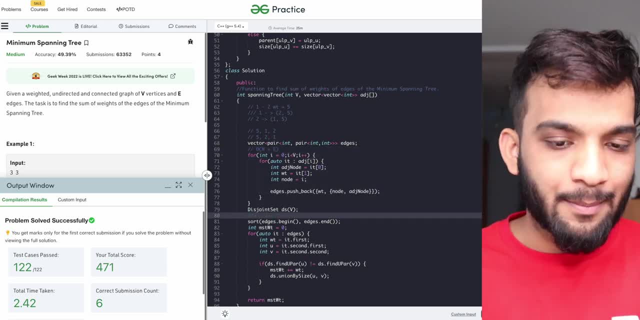 number of edges because you're going. number of edges because you're going across. right then you're sorting it across. right then you're sorting it across. right then you're sorting it. imagine you have images m logarithmic of. imagine you have images m logarithmic of. 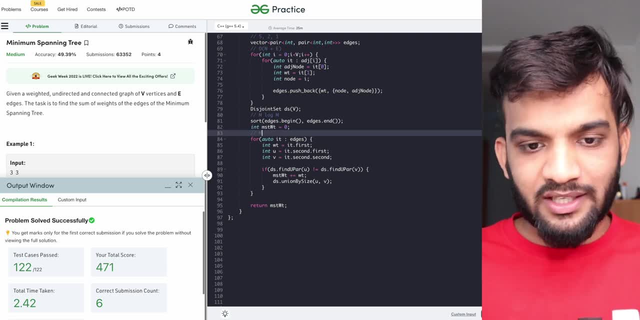 imagine you have images, m logarithmic of n? m to sort it, and then you're moving n? m to sort it, and then you're moving n? m to sort it, and then you're moving across all the edges and you're using a across all the edges and you're using a. 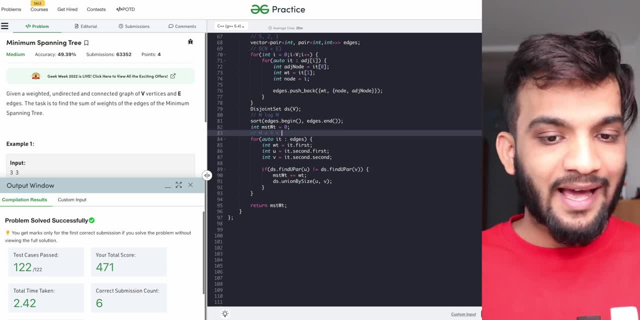 across all the edges and you're using a disjoint set data structure which we disjoint set data structure which we disjoint set data structure which we know is four cross alpha. so we can write: know is four cross alpha, so we can write: know is four cross alpha. so we can write it as m cross four cross alpha. and what? 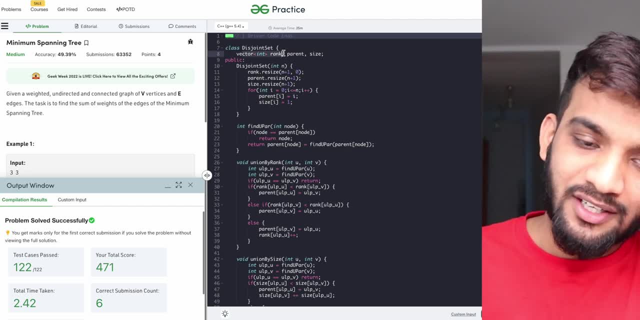 it as m cross four cross alpha and what it as m cross four cross alpha. and what uh external space? am i using this uh external space? am i using this uh external space? am i using this? disjoint set data structure will be. disjoint set data structure will be. 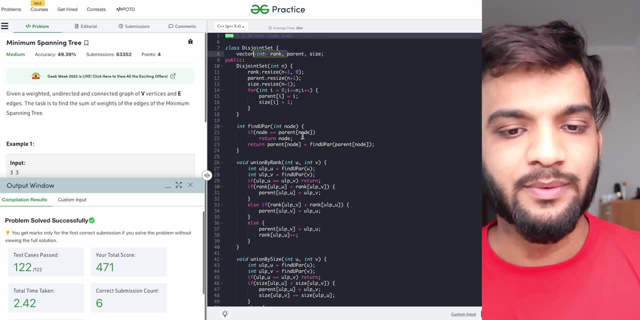 disjoint set data structure will be using a parent and a size. you can omit using a parent and a size. you can omit using a parent and a size. you can omit the rank because we are not using union the rank, because we are not using union the rank, because we are not using union by rank. but yeah, uh, we're using a. 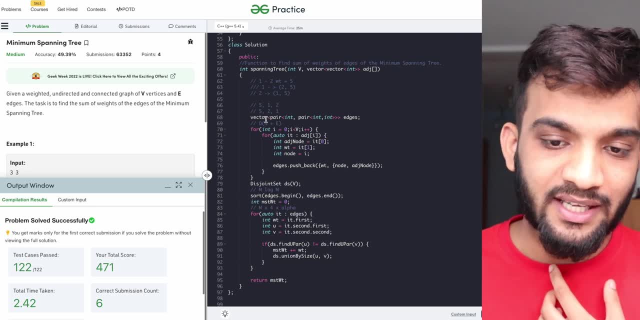 by rank, but yeah, uh, we're using a by rank, but yeah, uh, we're using a parent and a size that is the extra parent and a size that is the extra parent and a size that is the extra space, and we are using an extra space, space and we are using an extra space. 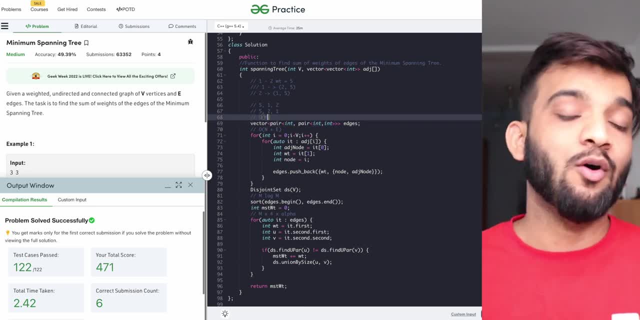 space and we are using an extra space to store, to store, to store uh edges as well, so we go off m over uh edges as well. so we go off m over uh edges as well. so we go off m over here. so these, uh, this is the time and 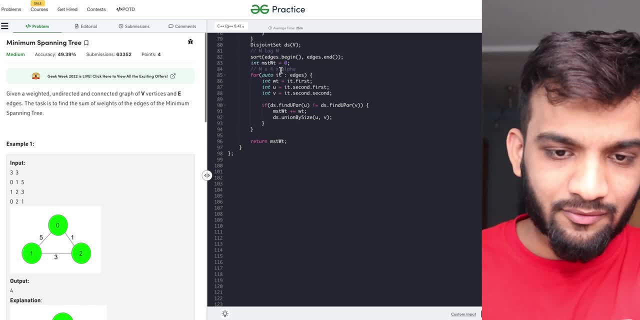 here so these, uh, this is the time. and here so these, uh, this is the time. and the space complexity, the space complexity, the space complexity i am using, if you carefully see, like four i am using, if you carefully see, like four i am using, if you carefully see, like four, alpha is used twice, so probably 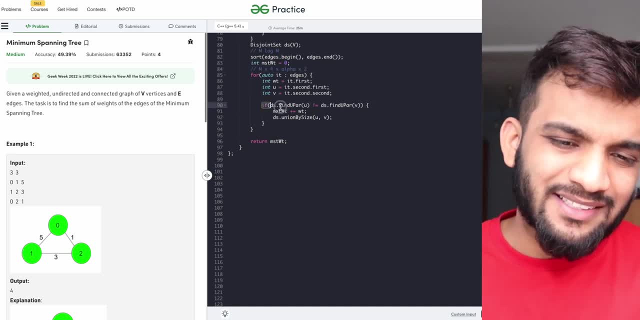 alpha is used twice, so probably alpha is used twice, so probably another twice you can add, because another twice you can add, because another twice you can add, because this will be executed very limited. this will be executed very limited. this will be executed very limited number of times. 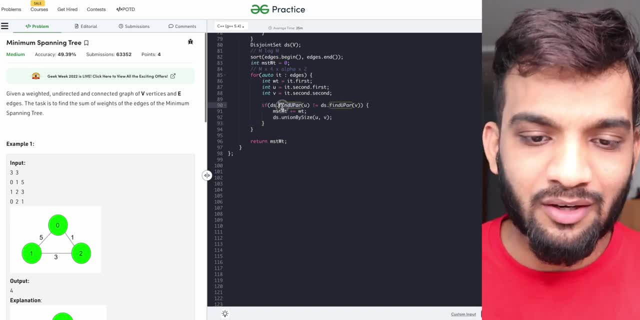 number of times. number of times like very, very rare case, uh, where the like very, very rare case uh, where the like very, very rare case, uh where the find you parent and union by size will find you parent and union by size will find you parent and union by size will always be executed. so yeah, for safety you. 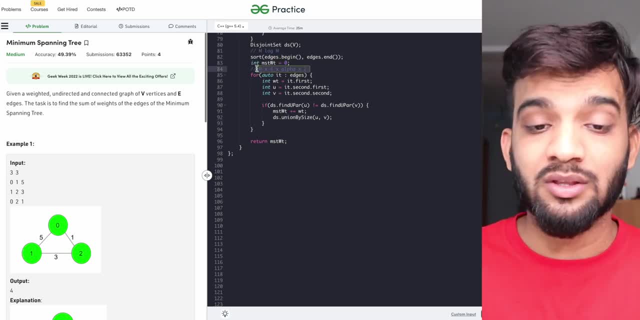 always be executed. so yeah, for safety, you always be executed. so yeah, for safety, you can just add a cross two because it's can just add a cross two, because it's can just add a cross two because it's twice. so this is what the time: twice. so this is what the time. 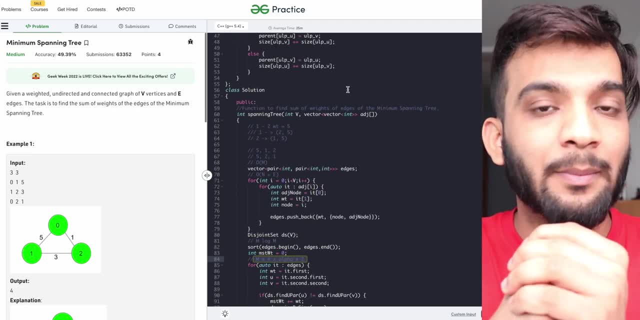 twice. so this is what the time complexity and the space complexity of complexity and the space complexity of complexity and the space complexity of truscull's algorithm is so guys, before truscull's algorithm is so guys, before truscull's algorithm is so, guys, before wrapping up this video, i would like to 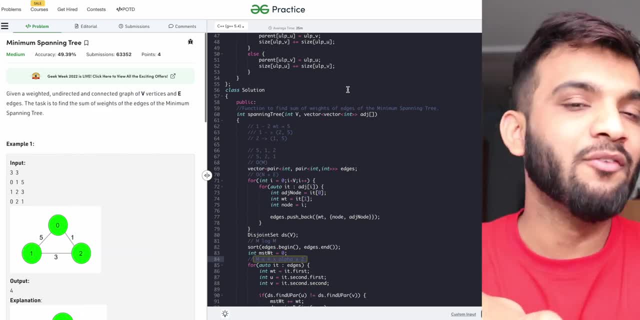 wrapping up this video. i would like to wrapping up this video. i would like to request you something as checking out, request you something as checking out. request you something as checking out our statistics- nearly 50 of the users. our statistics- nearly 50 of the users. our statistics- nearly 50 of the users who watch our video. do not subscribe to. 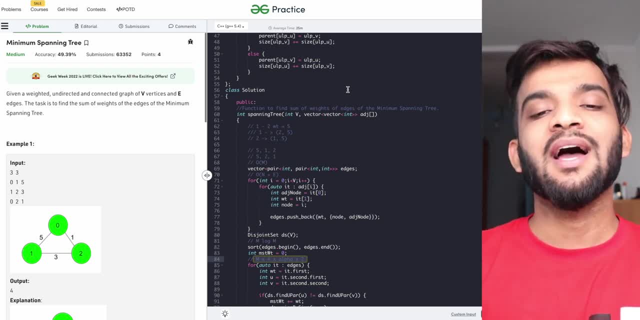 who watch our video do not subscribe to. who watch our video do not subscribe to us. so it's an earnest request that us. so it's an earnest request that us. so it's an earnest request that please hit that subscribe button. and if please hit that subscribe button and if 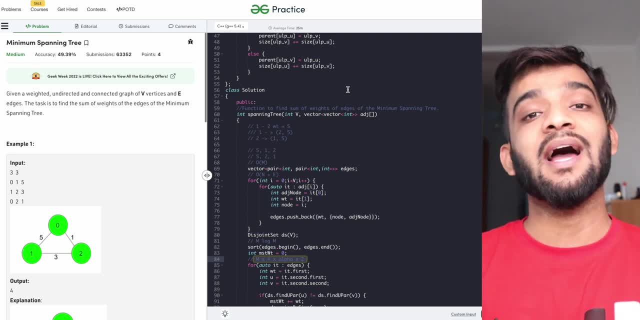 please hit that subscribe button. and if you understood the algorithm, the code, you understood the algorithm, the code, you understood the algorithm, the code and everything, do it that like button and everything. do it that like button and everything, do it that like button. and if you haven't checked out our dp. and if you haven't checked out our dp and if you haven't checked out our dp, series and the sd sheet, the links will series and the sd sheet. the links will series and the sd sheet. the links will be in the description, please make sure. be in the description. please make sure. be in the description. please make sure you check them out with this. i'll be you check them out with this. i'll be you check them out with this. i'll be wrapping up this video. let's put in some. wrapping up this video. let's put in some. 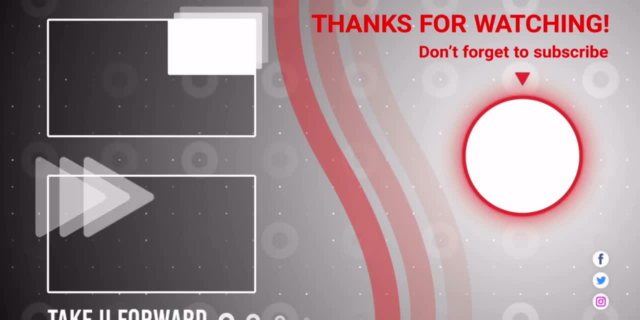 wrapping up this video, let's put in some other video. till then, bye, bye, take care. other video. till then, bye, bye, take care. other video. till then, bye, bye, take care. whenever your heart is broken, whenever your heart is broken, whenever your heart is broken, don't ever forget you're golden. don't ever forget. you're golden. don't ever forget you're golden. i will find a light. i will find a light. 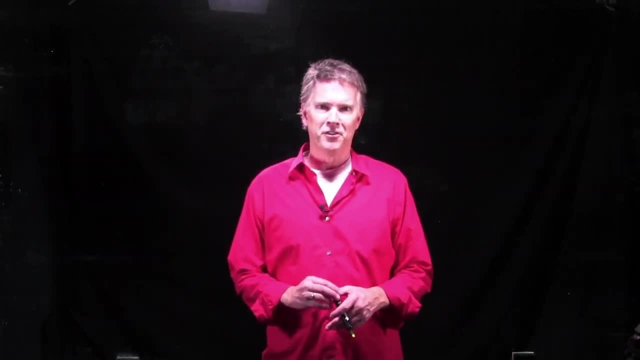 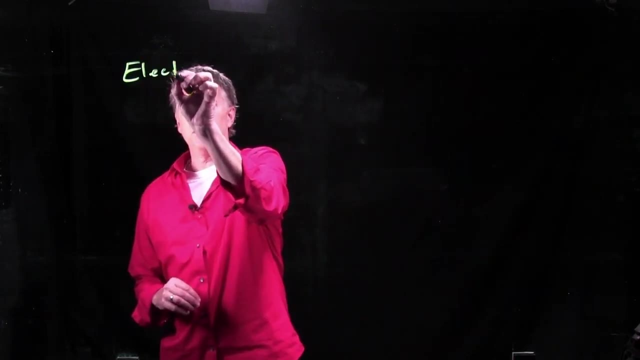 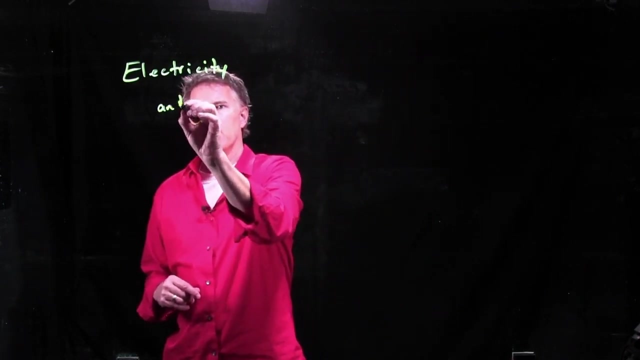 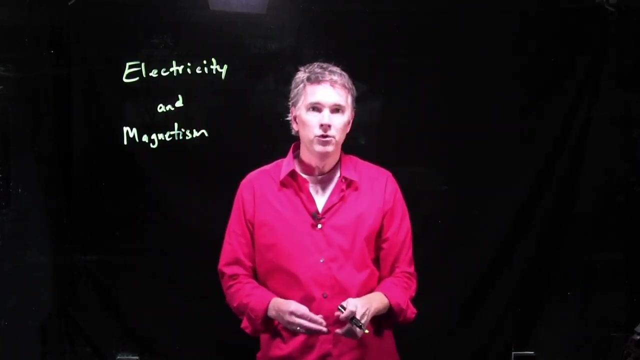 Hello class Professor Anderson. here We're talking about electricity and magnetism. this term It should be very exciting. Electricity is something that you have all heard of, of course, and you've probably also heard of magnetism. Well, it turns out that those are not two separate things, but in fact both part of the same thing. 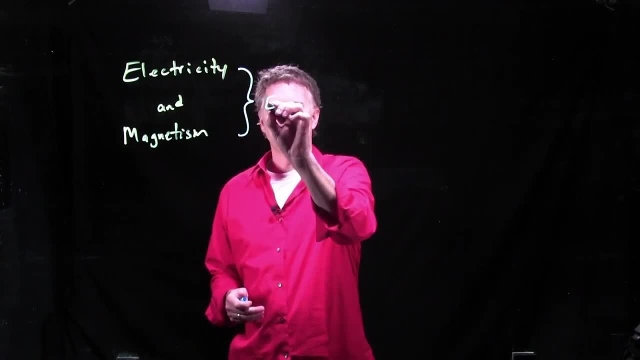 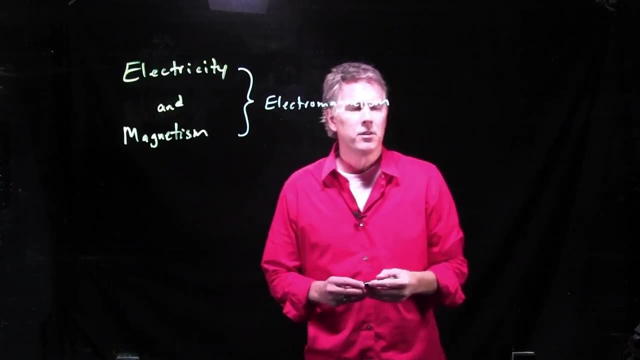 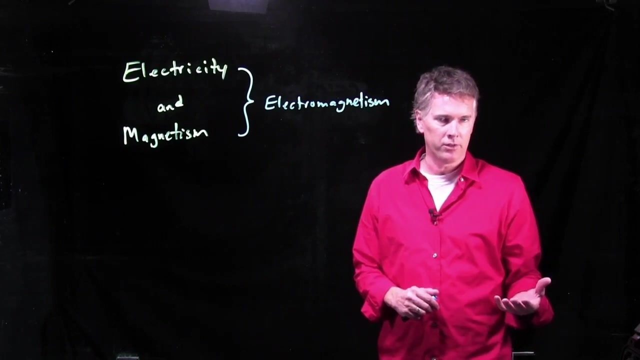 which is something called electromagnetism, And we're going to talk a lot about. what does electromagnetism mean? what does it mean for the universe around us? how does it affect the atoms and molecules and charged particles that are moving around in the universe?